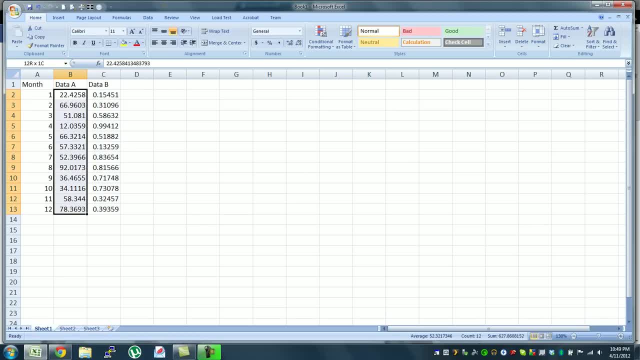 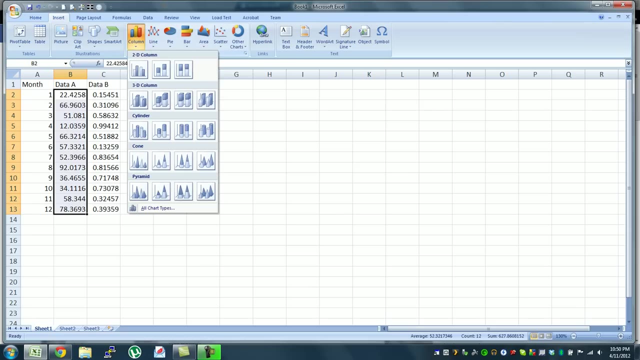 Two different types of data. We have whole numbers here and then we have numbers that are less than one here. So what we're going to do is start off by plotting our first set of data, data A- I'm going to highlight B2 through B13, go to insert and I want to make this a column. 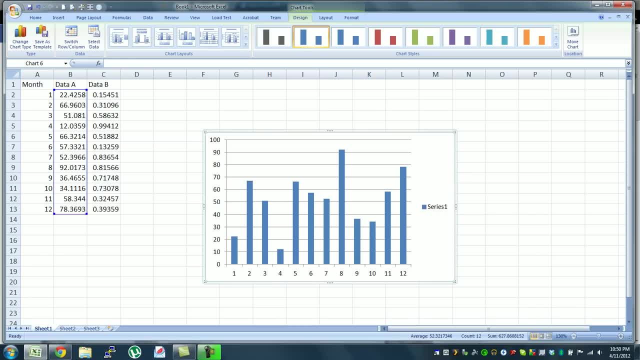 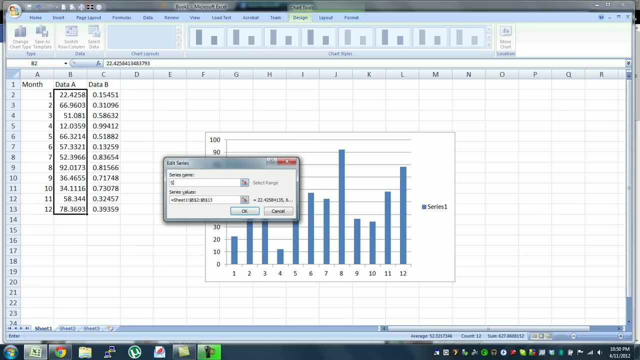 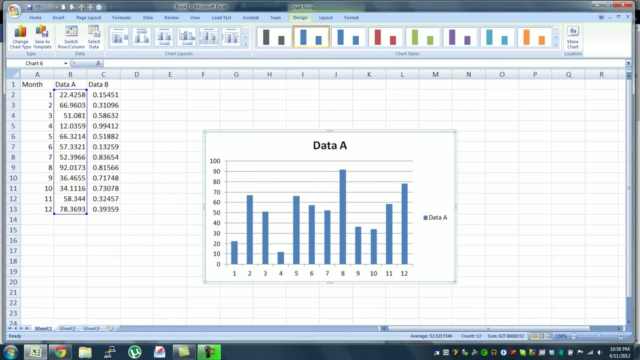 Pretty simple stuff. I'm going to change this from series 1 to data A by hitting select data. I'm going to edit this. call this data A. So now we have one series of data plotted. What we want to do is bring in the other set of data which tells the other side of the story. 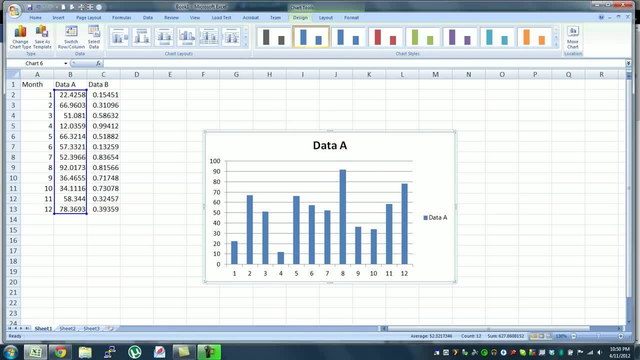 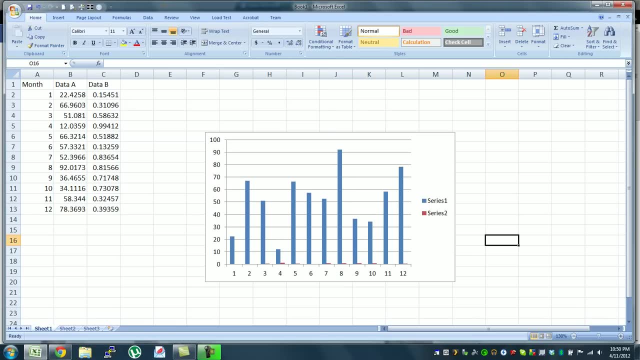 Pretty simple. What I'm going to do is, if I hit the corner of this box and drag it over, it's going to bring in series 2. But it's not going to graph it properly. So what we have to do is click on the series 2 so it highlights the box around series 2.. 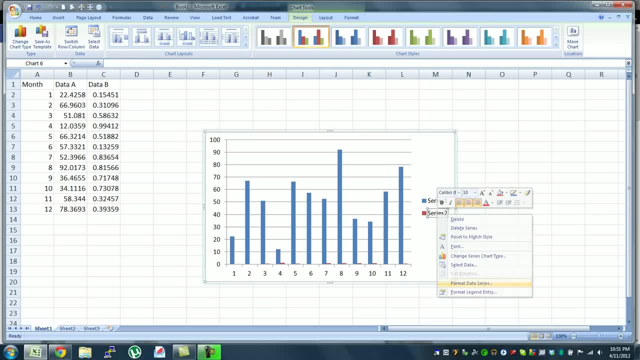 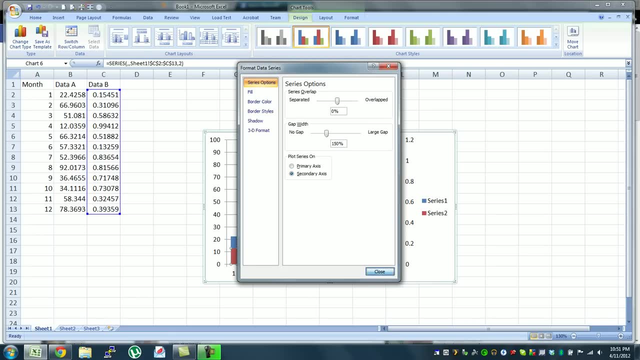 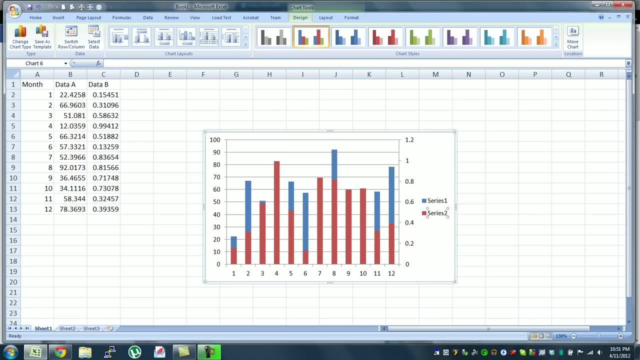 Right click. I'm going to go to format data series And I'm going to plot the series on a secondary axis. Still doesn't look right to me because it's not what I want. So for series 2, I'm going to change the chart type to a line graph. 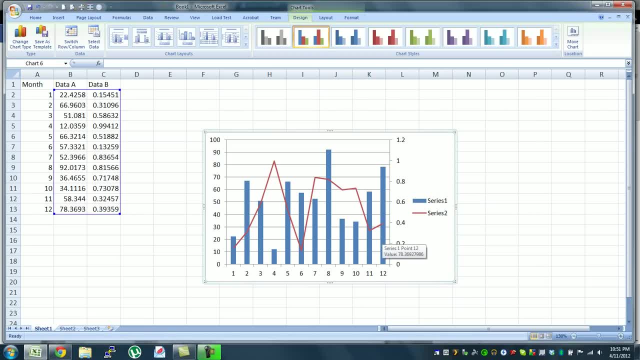 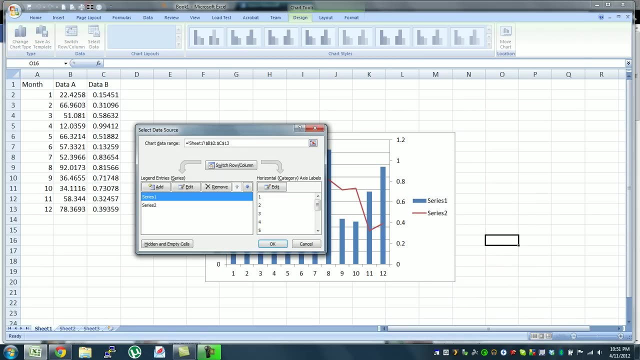 And now we're telling a different story here. So here we're able to see series 1 as a bar graph and series 2 as a line graph. If we want to change these names, you right click select data. series 1 is data A, so we're going to call that data A. 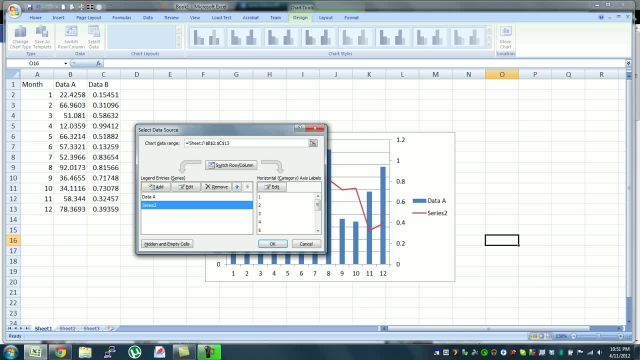 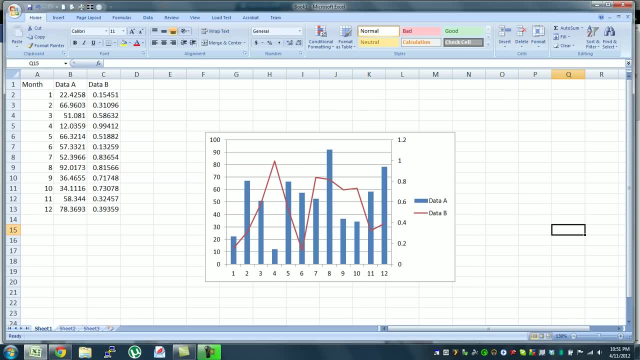 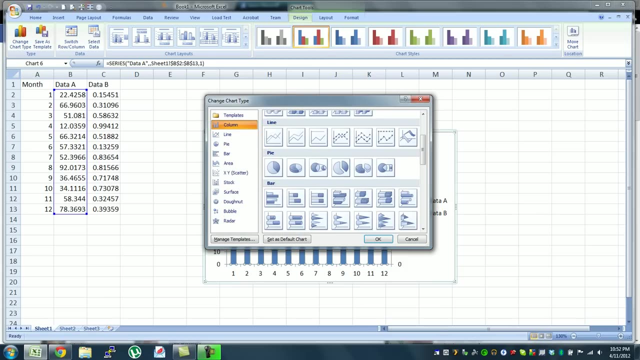 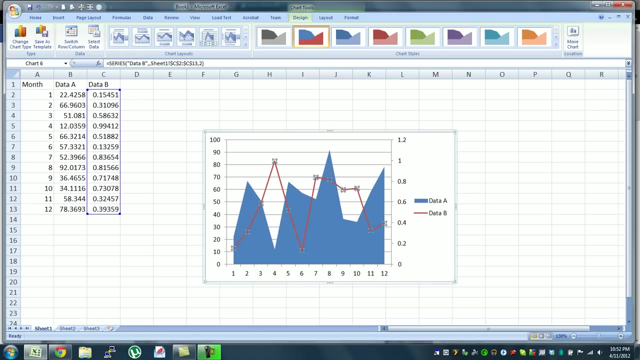 And series 2, we know, is data B. We can always go back and change this to, let's say, a mountain graph Area, And we can change data B to our bar graph. Either way, it's whatever helps you tell your story the best. 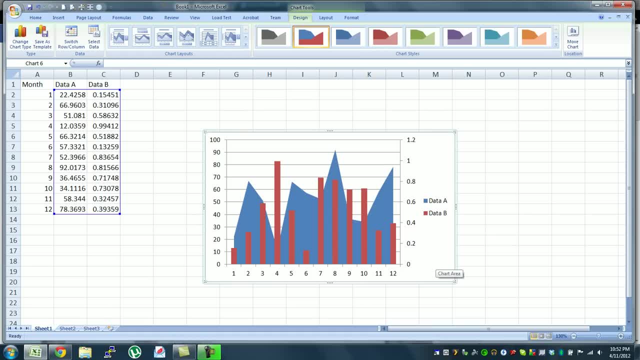 I hope you guys got a lot out of this. If you guys have any questions, head over to xlsxhelpcom and post your questions or comments there. Thanks guys.